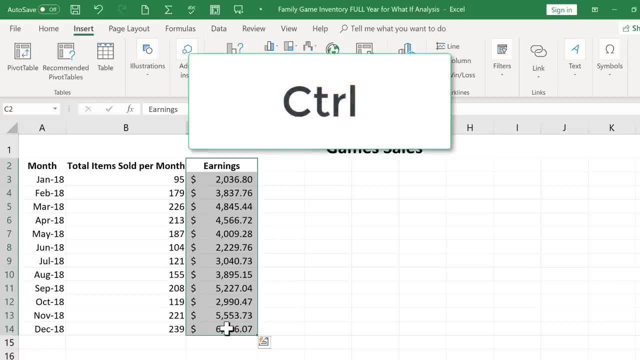 would like charted. Next, I'm going to hold the control key on the keyboard and now I'm going to move my mouse over here to column A and, still holding the control key, I'm going to click and drag from the word month all the way down to the bottom of the data. Now I can release the control. 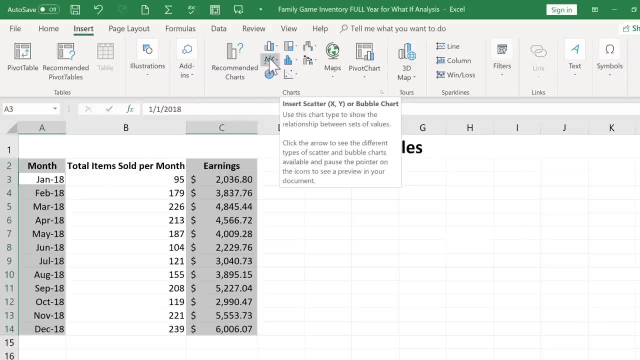 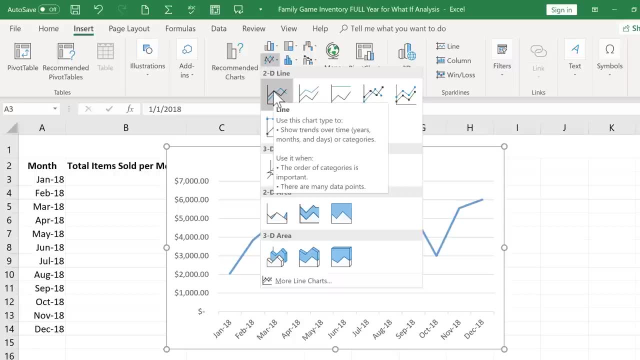 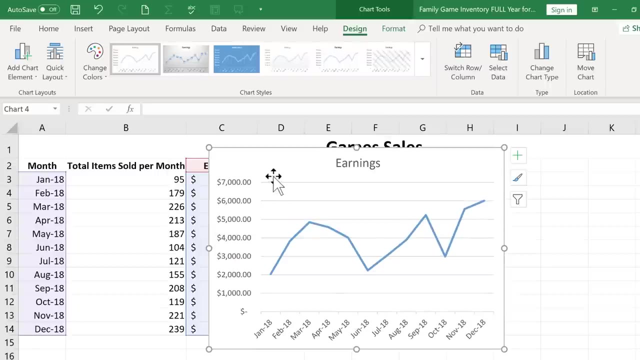 key. Now I can simply go up here to the charts group and select line chart. There's a bunch of different ones I could choose, but I'm going to stick with this particular kind here line chart. I click it and it shows me a nice chart of the earnings for this small business. 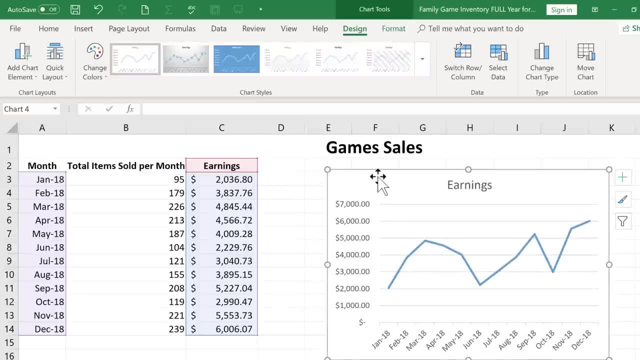 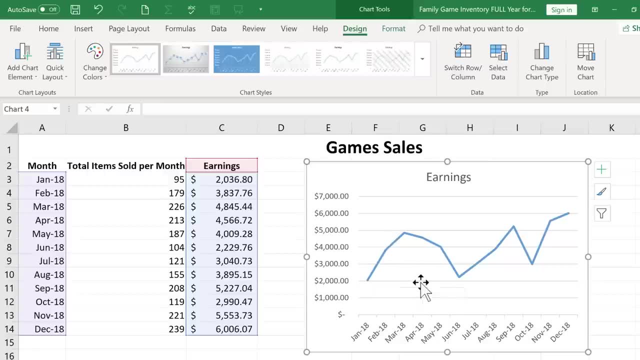 I'm just going to move that chart over to the right a little bit and let's take a look at it. So this gives me some good information about the trends, at least the trends as of 2018.. You can see that the earnings are building somewhat over time, but there are these dips. 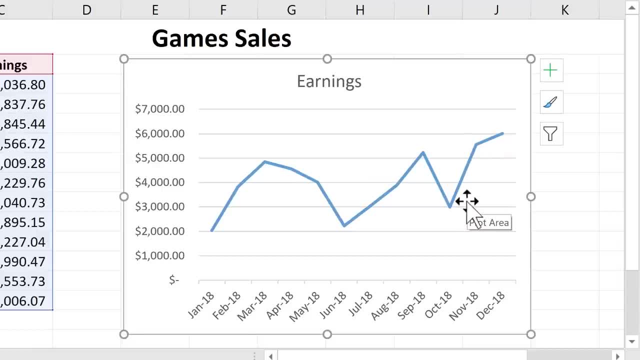 as well. So to help us get a sense of where things are headed, something we can do is click on the line. When you do, you can see that it highlights the line and it also highlights the different data. each of these points is an earnings amount from the data here at the left. Now I can carefully. 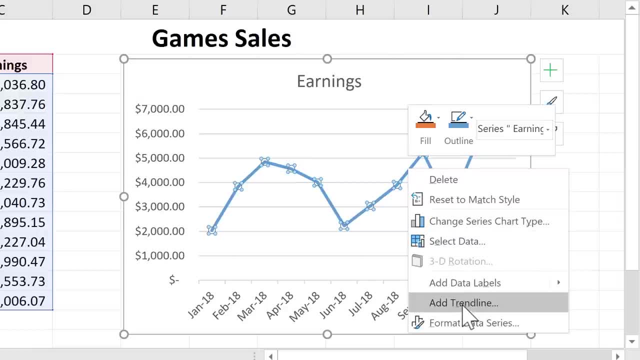 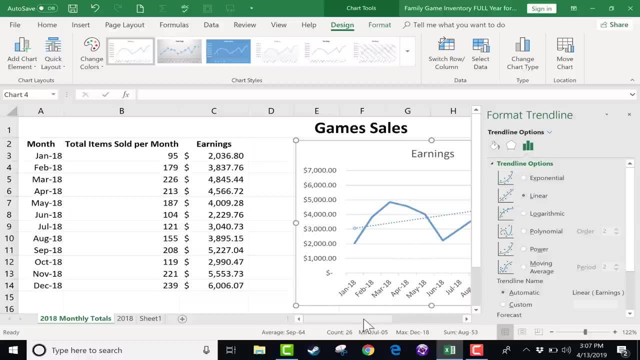 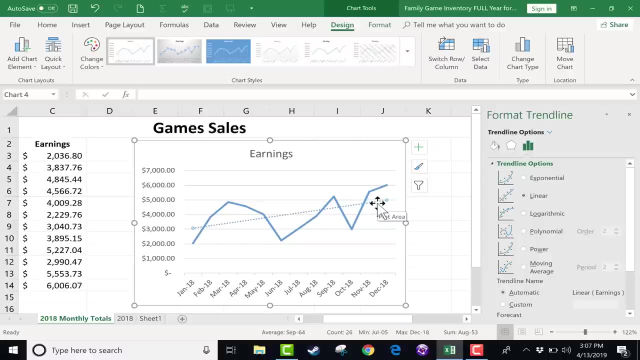 right click on that line and choose add trend line. Look what happens when you do that. First of all, you get a panel that opens on the right, and if I scroll horizontally a little bit, you'll be able to see this better. You can see that a trend line has been added to my chart. 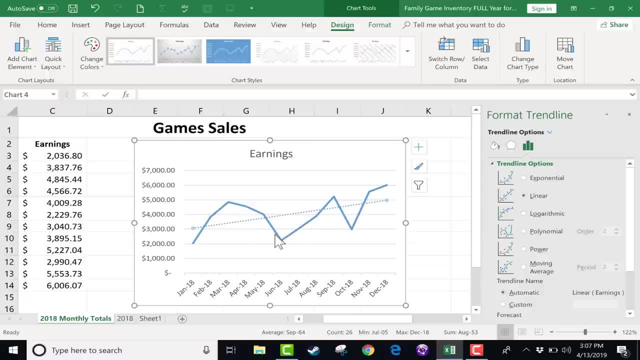 So this helps me get a sense of how things are trending. Even though there are ups and downs, it looks like it's going to be a trend line, So I'm going to click on the trend line and I'm going to click on the trend line. You can see that the trend is gradually up. Now let's look at the panel. 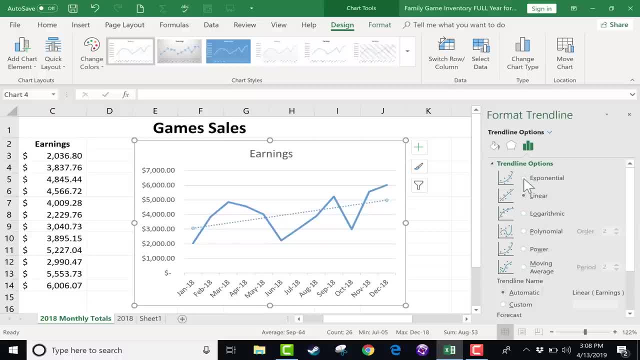 that opened on the right side, You can see that there are different options here. For example, there's exponential Instead of linear trend line. you could do an exponential trend line And, to be honest, I don't totally understand the difference between the two, other than exponential is more. 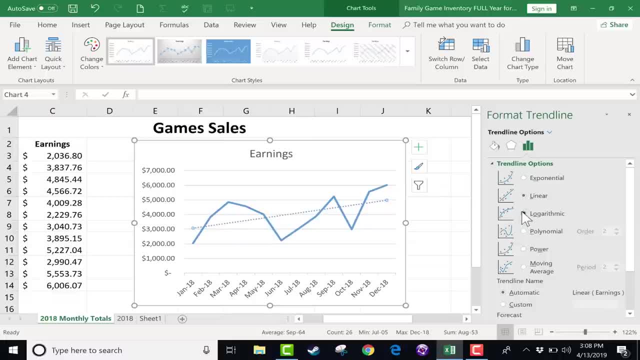 curved and linear is straight. There's also logarithmic polynomial and I think these are all basically statistical trends. So let's look at the chart. I'm going to click on the trend line and I'm going to click on the trend line and I'm going to click on the trend line and I'm going to click on the trend line. 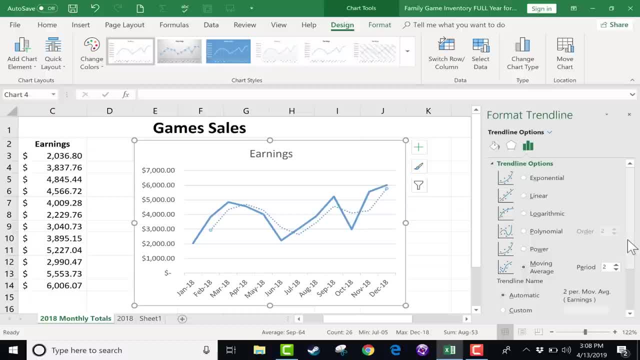 I'm going to click on the trend line and I'm going to click on the trend line. So if you've taken statistics, you probably understand this part much better than I do And I think I'm going to stick with linear, With linear selected. if I browse down the panel a little ways, look at what I can. 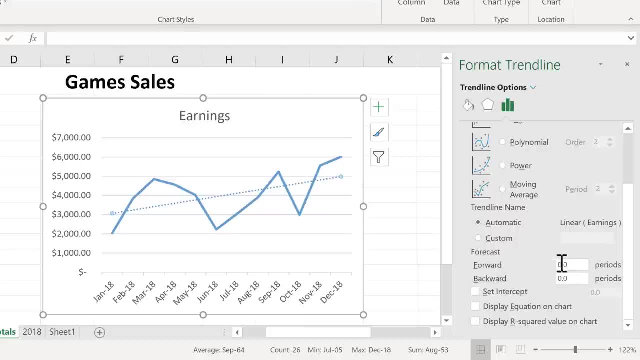 do. There's a forecast option and I can forecast forward, let's say, five periods. I tap, enter on the keyboard and you can see what that did. It adjusted my chart to include a forecast of five more months. I could change that to, let's say, 20 periods. Let's look at that. So now you can see. 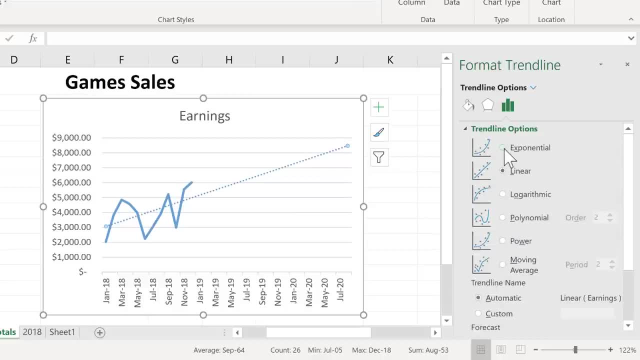 that trend line and how it's dramatically going up. If we change it to exponential, it looks similar, but there are some differences. Now, as you're doing this, as you are looking at trends and future forecasts, notice that there are some other options. down here There's a set intercept. 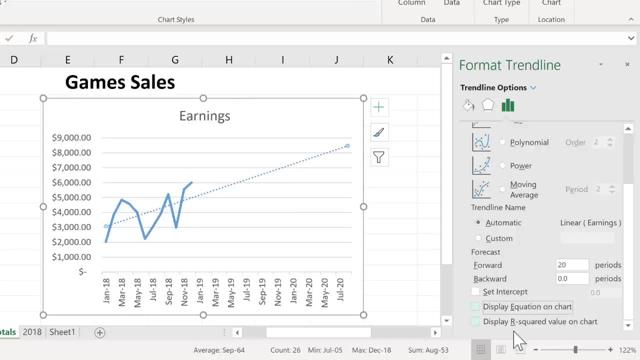 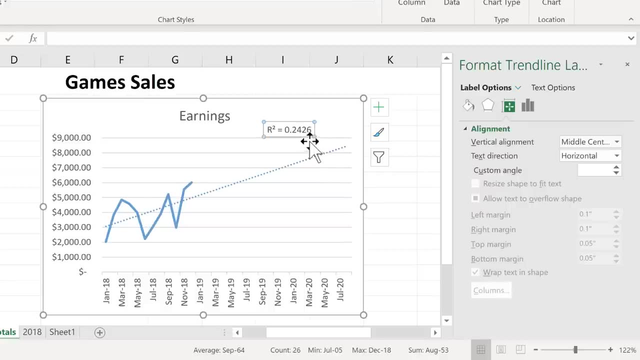 If you understand what that means, go for it. There's a display equation on chart and there's a value on chart And my understanding is that this r-squared number has to do with the accuracy of the predictions. Notice that there are some trend line options, For example. you can add some. 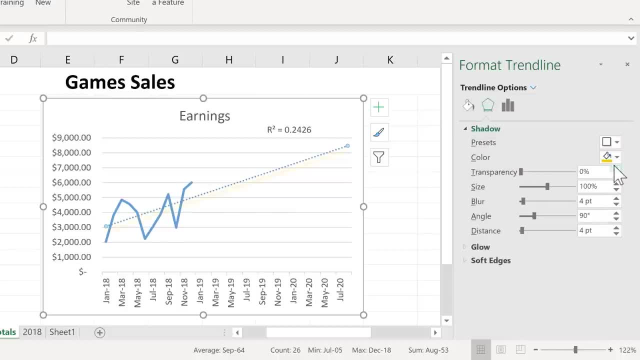 effects. If you want to put in a shadow, I just put in kind of a peach-colored shadow. You can put in a glow. I mean, we can really make this pretty fancy if we want to. I'm actually going to take that off. And there are also some color options. I can change it to, let's say, yellow. I can change. 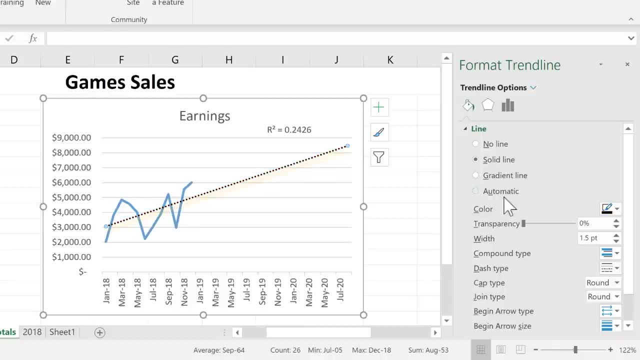 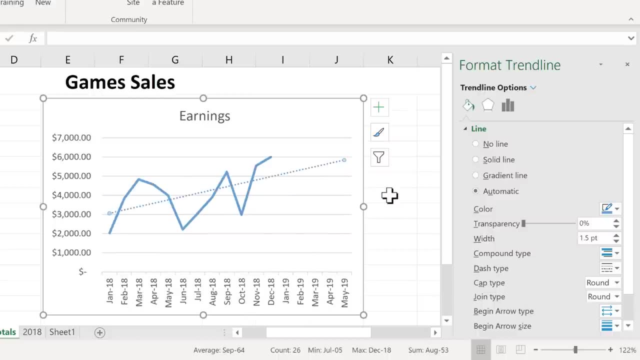 it from blue to red to black, whatever color I want that line to be. At this point, I'm going to undo all of this work that I've just done and go back to before I put the trend line in. I'm just 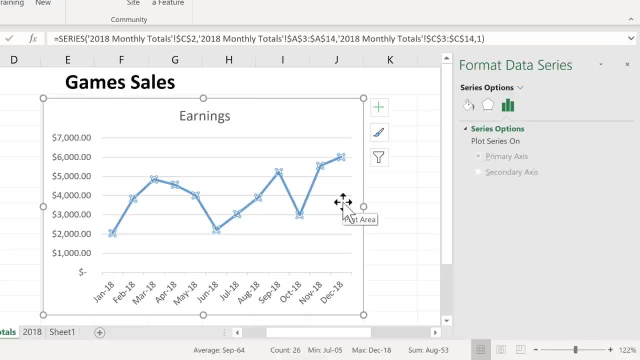 holding ctrl and tapping z to undo. Next, I'd like to show you how you can add that same trend line, but do it directly in the spreadsheet, using Excel functions. Now, why would you ever want to do it this way? Well, for one thing, it enables you to change the color of the trend line If you want to. 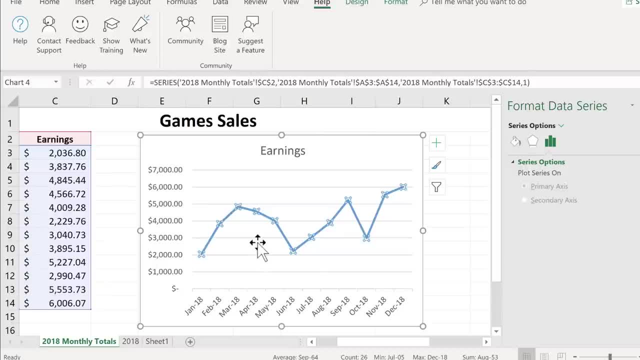 change the color of the trend line. you can do that in Excel, But it also enables you to actually track more than one type of trend line, And you'll see what I mean in just a minute. And there are other reasons as well why you might want to do it this way. So I'm going to scoot this chart to the 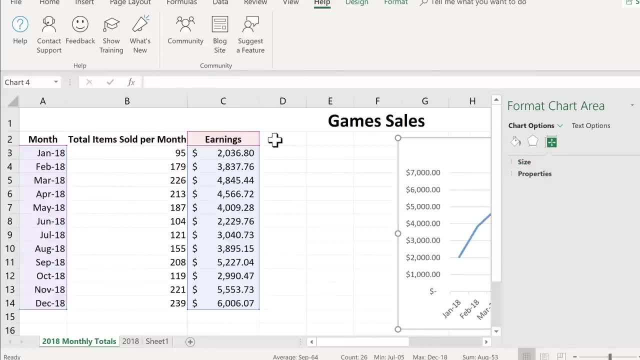 right, just a little bit, And I'm going to come over here next to earnings, And I'm going to type here trend forecast, here at the top And next to that growth forecast. So I just tap enter And it looks like the text did not fit. So I'll just click and drag it And then I'm going to 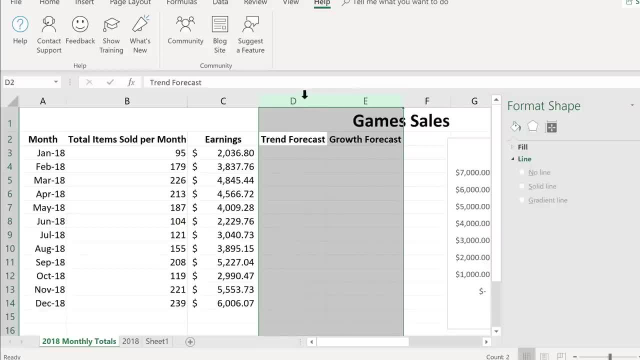 drag to highlight both of those columns And then just double click between them, And it should expand them out so that the text fits perfectly. The next step is kind of tricky. Now, before I do this next step, we need to think about this. What I'm about to do is create a formula that looks at 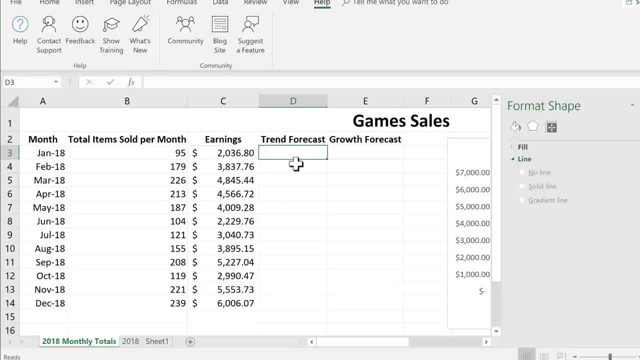 the trend of this data. And, if you think about it, a trend cannot rely just on one cell, one piece of data. That doesn't make sense. How can you have a trend based on one thing? And so for that reason, I can't just select cell D3 in this case, and type in my formula Instead. 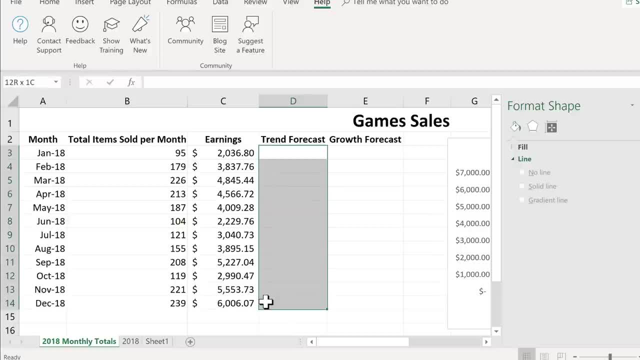 I have to click and drag to highlight the entire range to the right of my data. Next I'm going to type equals, So this range basically equals. I'll type the word trend and then left parenthesis, And then I'm going to select the data that I want the trend to be based upon. So I click and drag. 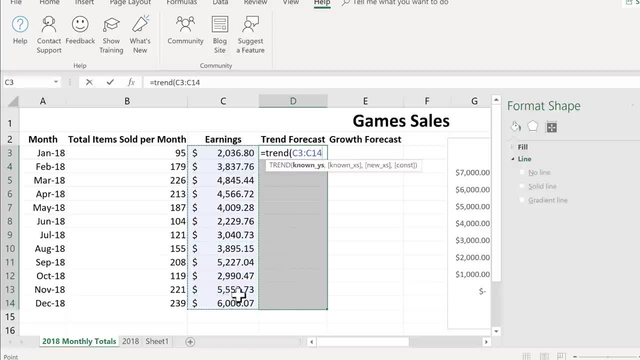 to select this entire range. Next, I should put in the right parenthesis, but I don't have to, so I'm not going to Now think about it. Typically, when you put a formula into a cell, when you're done, you just tap enter. 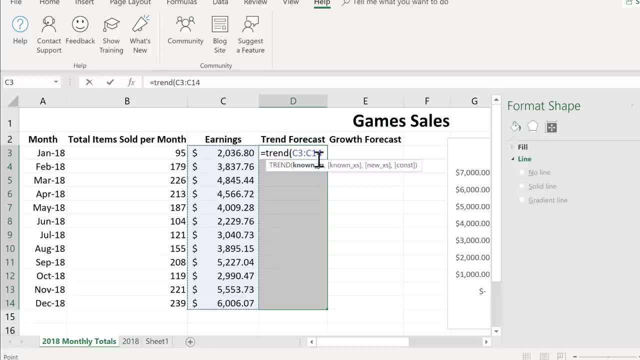 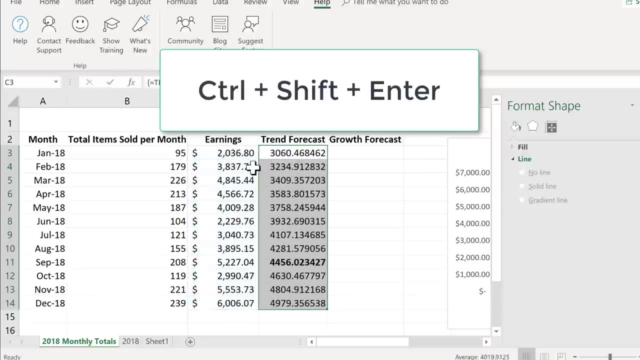 But in this case you can't. The reason why is because this data is dealing with an array. It's dealing with more than just one cell or one column. It's a whole array. So instead of tapping enter, what you need to do is hold control, hold shift and then tap enter And look what it did. 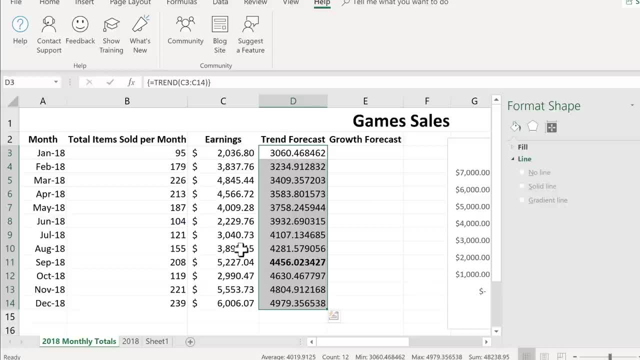 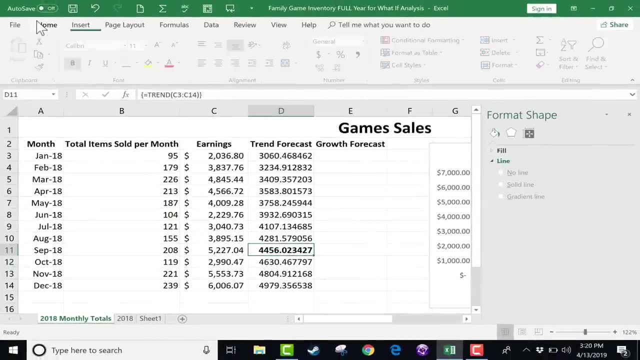 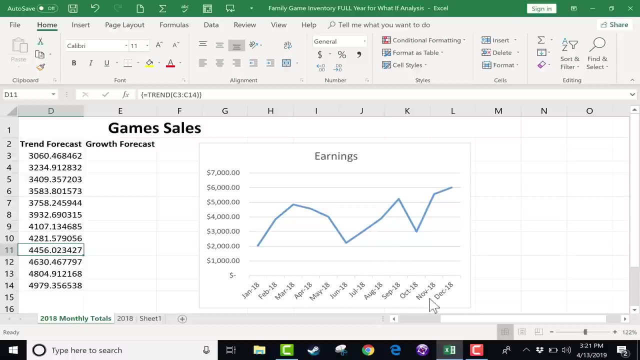 It created some trend data Based on these numbers here at the left. this is the trend. Now, for some reason, it put this particular cell in bold. I don't know why. I'm going to take that off. So now, if we go back and look at our chart, nothing's changed so far. So now I'm going to redo this chart. 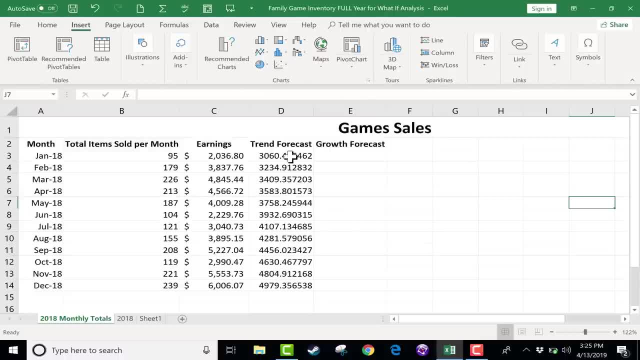 I'm just going to delete the chart out And once again I'm going to click and drag. And this time I'm going to click and drag to highlight both earnings and trends, And then I'm going to click on forecast columns, Then I'll hold the control key and select month. 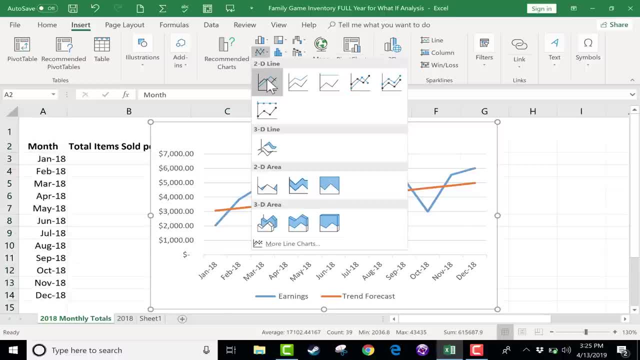 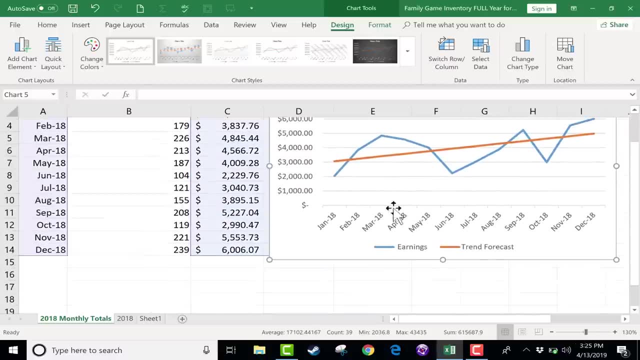 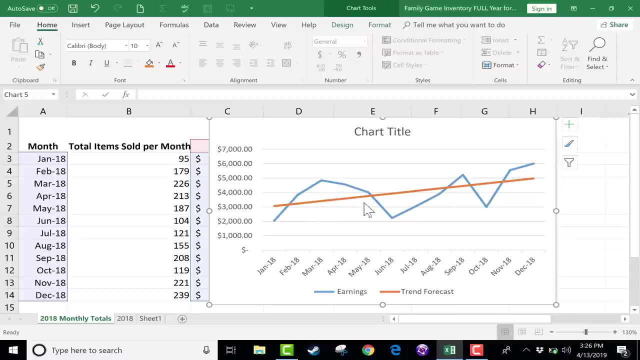 Now I go up and select that same line chart right here And take a look at that. The chart now incorporates both my data of the earnings and also the trend line that was calculated using the trend function. So that's kind of nice And I really like the different colors that come in. Of course, you. 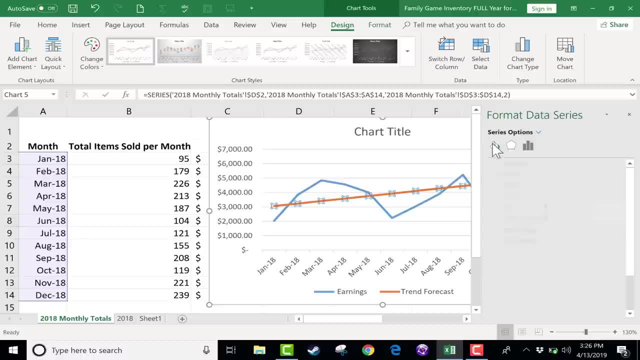 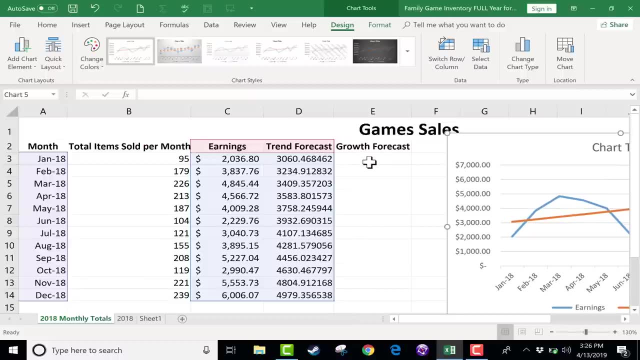 can change those colors. just by selecting a line, You can go in and change the color that it has. Now, the last thing I'd like to show you here is you can do a similar thing if you want to show an exponential forecast. And again, I don't totally understand the differences between the two. 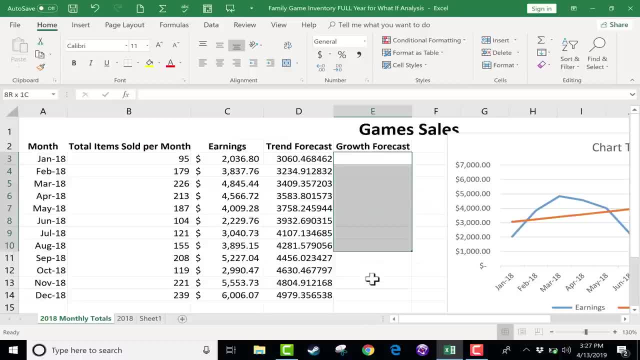 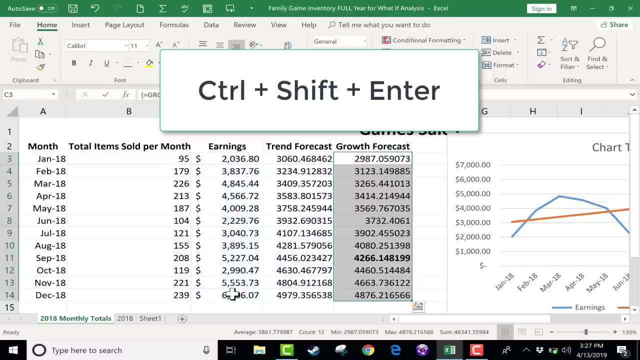 So in this case, just like before, you would click and drag to highlight the whole range- type equals growth, left parenthesis, and then select the data that it's going to be based on. I want to tap enter on the keyboard, but that's not right. I have to hold control, shift and then enter. There's my data. 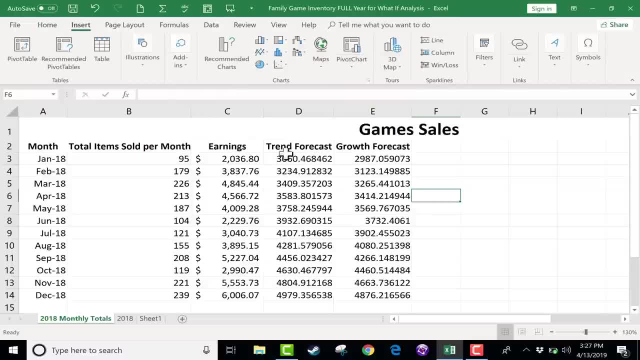 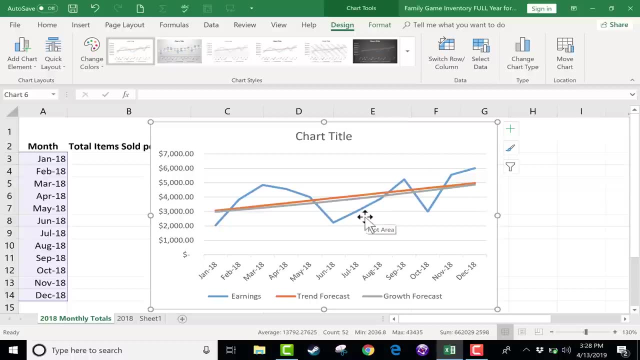 Now, if I create that same chart again, this time clicking and dragging to highlight all the data I want included, and then hold control because I don't necessarily need the items sold, I'll just go here to month and I'll click and drag to get month, go to that same chart and click. So now you can see three. 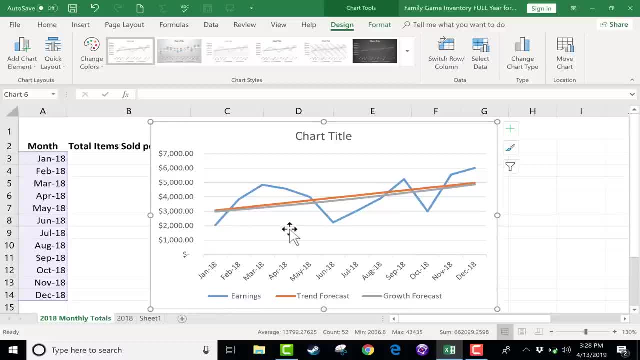 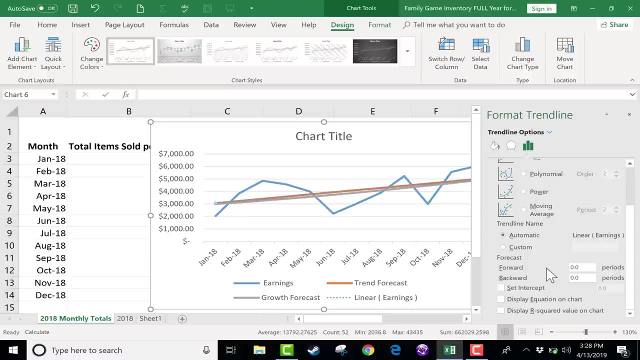 separate lines, each one marked differently: Earnings in blue, trend forecast in orange and the growth forecast in gray. When I right clicked to add a trend line, it gave me the option of looking ahead. looking forward five months, 10 months, 20 months. So what if I wanted to do that with this other method that I 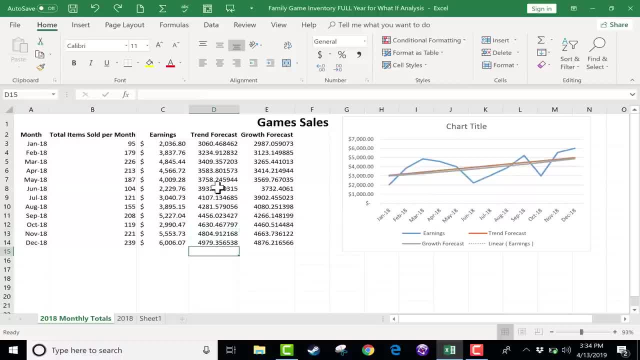 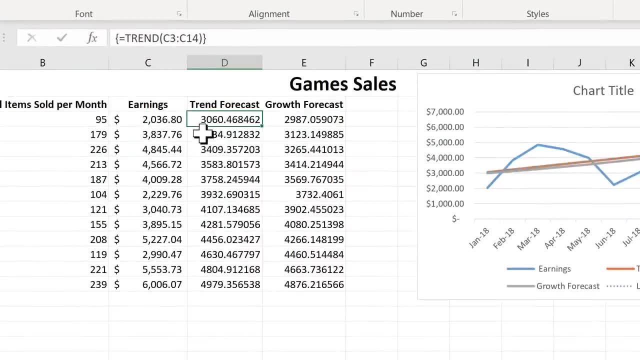 just showed you, of using an Excel function. To do that, we're going to have to first change this data. So this data here, if you look carefully, it's actually based on formulas. We need to change it to values only, And one way to do that is to click and drag to highlight the whole range and then put 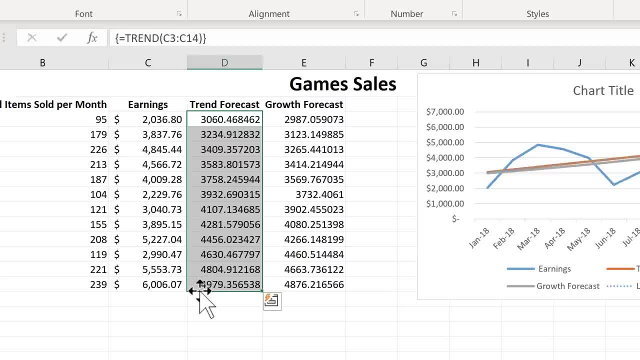 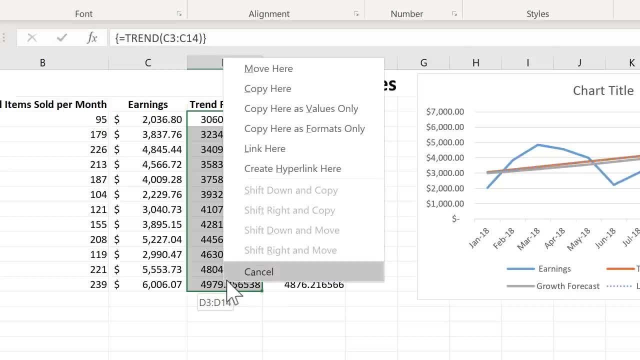 your mouse at the very bottom edge of that range and right click and just drag down a little bit- or left or right, doesn't matter- and then right back on top of itself. And the way Excel interprets that is that we want to copy this data back on top of itself. However, this time we're going to copy as: 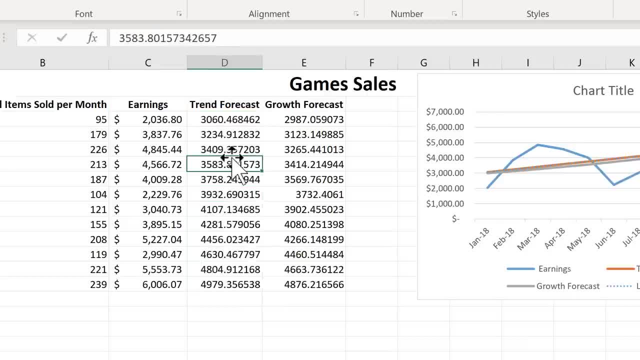 values only, So I select that. So now if I click here, you can see this is not based on a formula, it's just numbers. Let's do that also with the growth forecast. So I'll click and drag. highlight the whole thing. put the mouse at the. 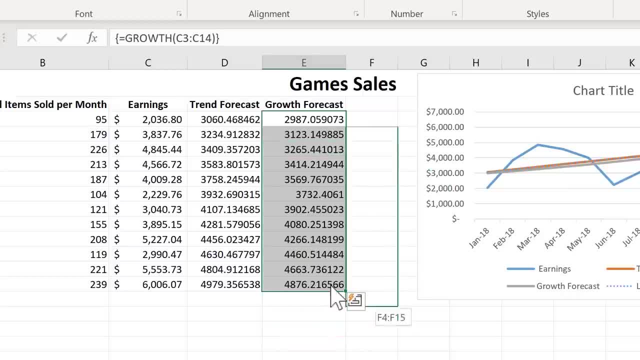 very bottom edge, right, click, drag down or right wherever I want to go, and then right back on top of itself, Copy here as values only. So now I can click and drag to get that whole range and I can go to the lower right corner of the range. You can see the autofill handle is there, If you've watched. 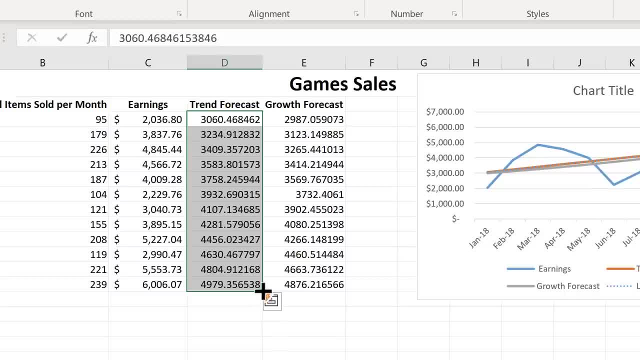 my previous tutorials. you know all about the autofill handle, But you put your mouse right on that and click and drag, and I'll explain how to do that in a little bit. So I'm going to click and drag and I'll. 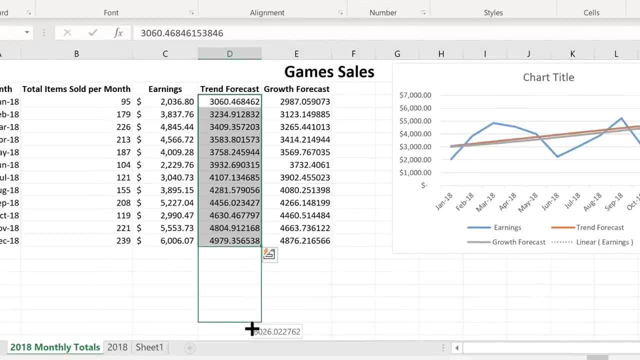 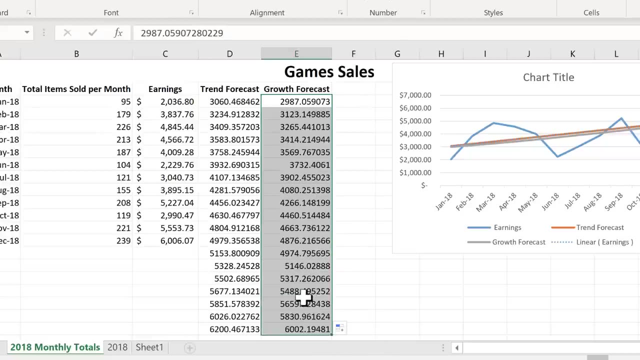 extend this out, maybe 5 or 6 more months, maybe 7.. I let go. and it's now making some forecasts based on the trend. Let's do the same here with the growth or exponential data, Lower right corner: click and drag down and there we go. And now I can also do a similar thing with the months to extend. 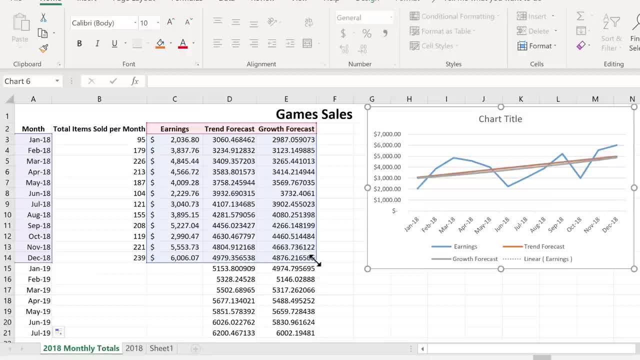 that out, And now, if I click on my chart, you can see what I need to do here. I need to extend this range down to include all of this new applied data that I created. I'm going to go ahead and mình new data in my chart, And there you have it. Now we have a chart that is based 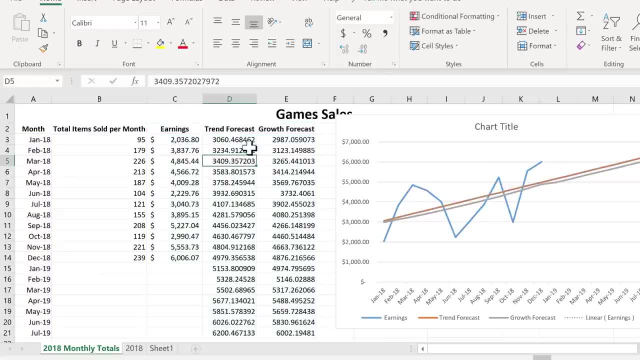 purely on the data in this spreadsheet. Yes, I did use a couple of functions- trend and growth- but this chart is dependent on the numbers here at the left. So we've looked at two different ways to create a chart that tracks recent trends and forecasts for the future. We looked at the much easier 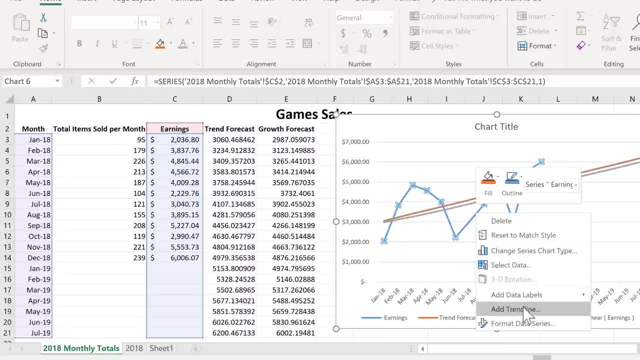 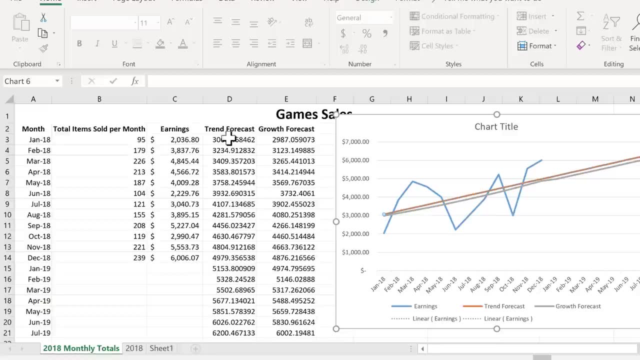 method of simply right-clicking on the chart and adding a trend line, and then we also looked at how to create that yourself using the trend function and the growth function. Thanks for watching. I hope you found this tutorial to be helpful. If you did, please click the like button below and consider connecting. 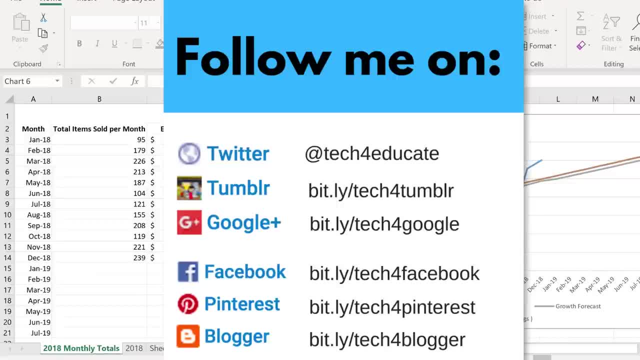 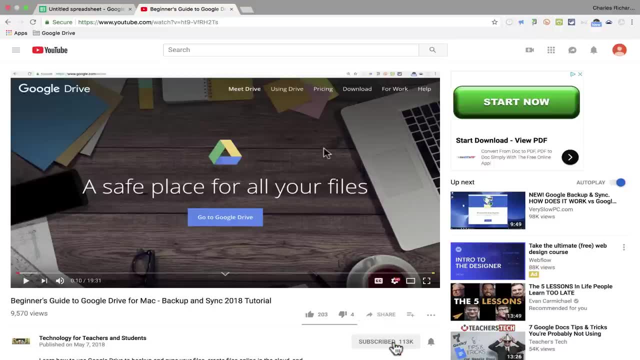 with me on my social media accounts like Facebook, Pinterest and Twitter, And definitely do subscribe to my YouTube channel for more videos about technology for teachers and students. And when you do subscribe, please click the bell next to the subscribe button. If you'll do that, you'll be notified whenever I post.